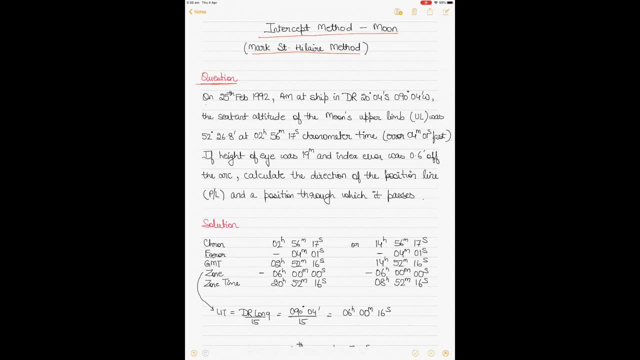 the question here. The question says it's 25th of February 1992 and it's am at ship. That means that it's morning on the ship and in the DR position, which is the dead reckoning position or estimated position. 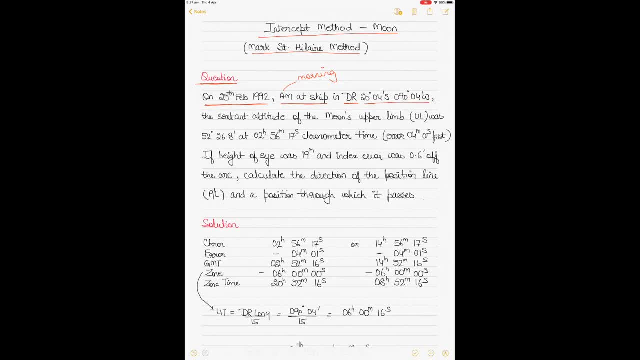 20 degrees 4 minutes south and 90 degrees 4 minutes west. The sextant altitude of the moon's upper limb, or UL, was 5226.8 at a chronometer time of 2 hours 56 minutes and 17 seconds, with a chronometer error of 4 minutes and 01 seconds fast If the height of I was 19 meters. 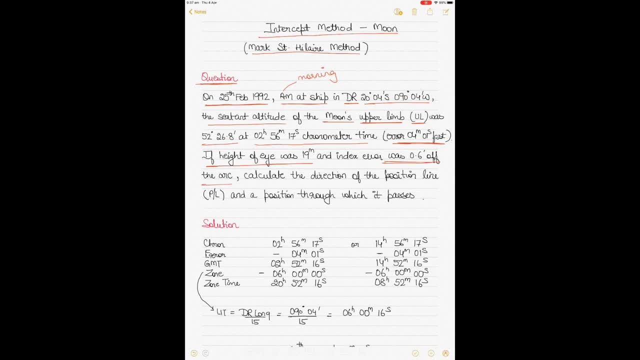 and index error was 0.6 of the arc. you have to calculate the height of the moon. Now I will explain the direction of the position line and the position through which it passes. All right, so sorry about that. So if I start with the solution, and before I start with, 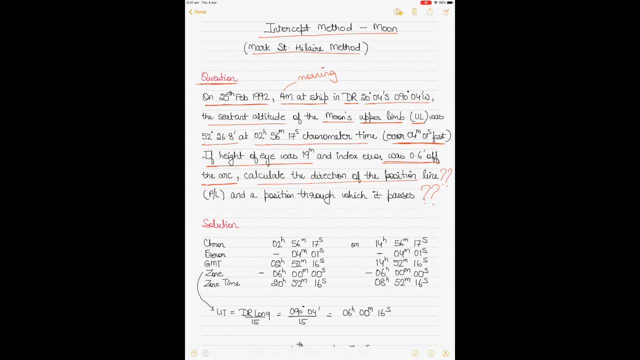 the solution. we have to solve something called the ambiguity of the chronometer time, And I have solved this ambiguity a number of times in my previous videos, but still, I'll take you guys through this. If you think that I rushed through it, please watch my other videos. Thank you for watching this. 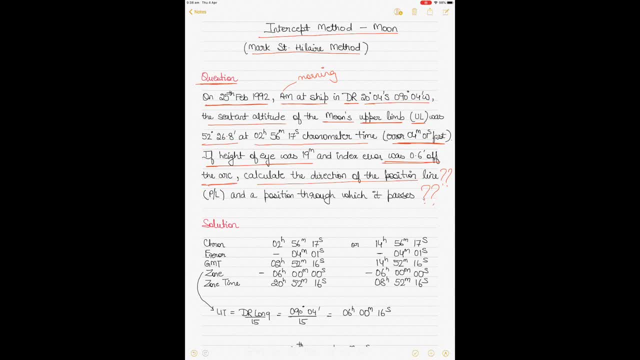 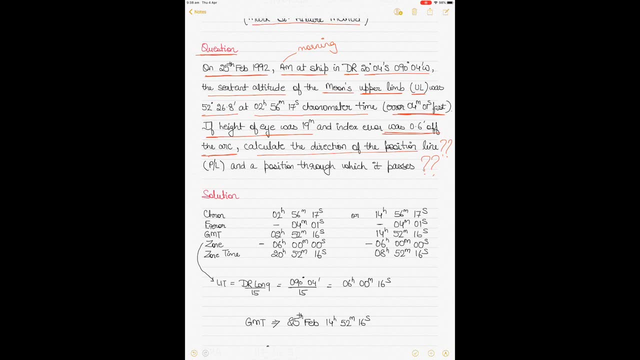 I hope you enjoyed this video and I will see you guys in the next one videos. and also there's a separate video titled ambiguity of chronometer time. you can watch that as well. all right, so anyhow, i'll quickly take you through this, as i have with my other videos. 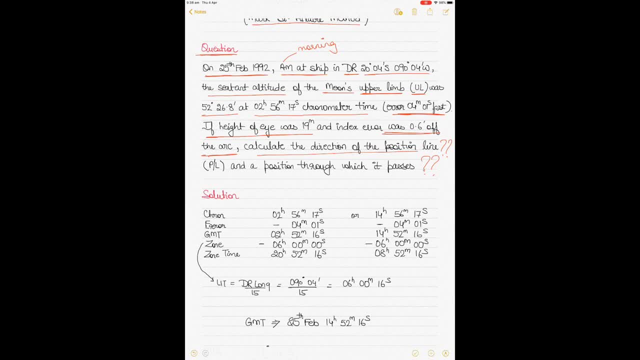 so whenever a chronometer time is given to you, you can have two scenarios with it. so you all have to do is, whatever time is given to you, just add 12 hours and write down another scenario, because when the chronometer shows 2 hours 56 minutes 17 seconds, it could be 2 in the morning. 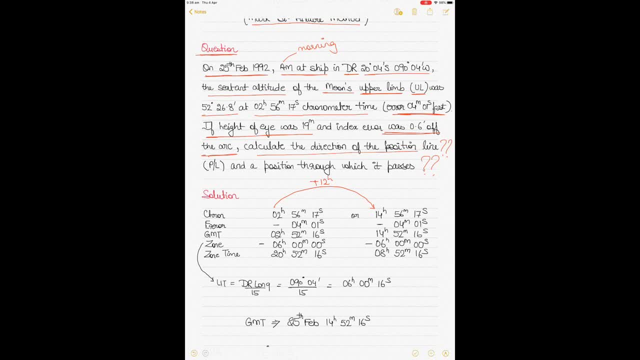 or 2 in the afternoon, which is 1400 hours, and because a chronometer looks like an analog watch and on your ship you don't know what exactly is the time at the gmt. the chronometer actually is a device on the bridge which gives you the gmt time. so when you look at the gmt time you could 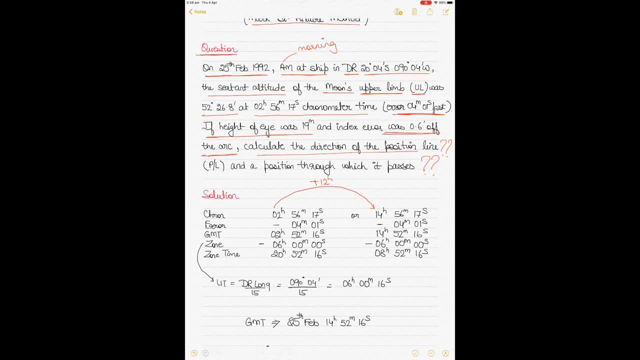 be on a very different longitude based on the gmt, and so you don't know what exactly is the gmt time. is it 2 in the morning or 2 in the afternoon in comparison to your position at the ship? all right, so in in your position. depending on your position or your longitude, it could be morning on your. 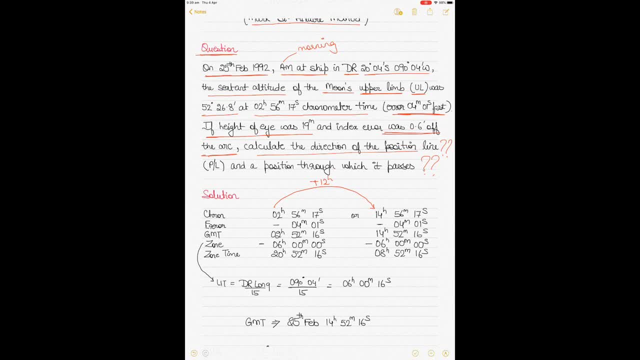 ship, it could be night at the gmt or vice versa, so we have to figure out from the chronometer time. so, anyhow, whatever the chronometer time is given to you, just add 12 hours to it and then write down both the scenarios and then apply your chronometer error. the same error is applied in both cases. 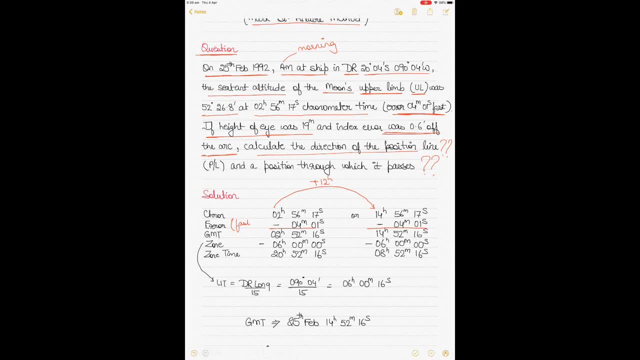 because the error is fast. that means chronometer is running ahead of gmt. we will subtract the error in both the cases. then you get two scenarios of the gmt time, and to figure out which is the correct scenario you have to apply something called the zone correction. now the zone correction is obtained from the longitude in time or lit. 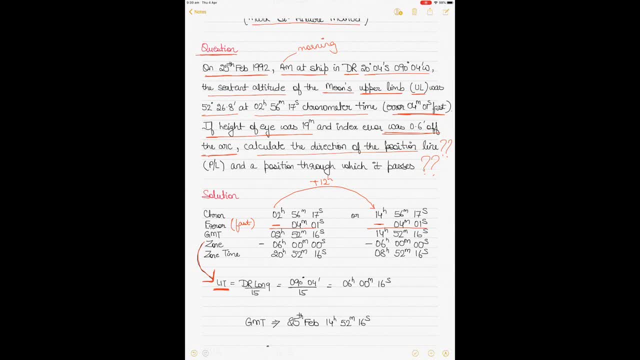 lit stands for longitude in time. that means every ship should have its own time based on its own longitude, which is not the practical way of time keeping, and that is why we use a correction called zone, which is the more practical way of time keeping. a zone refers: 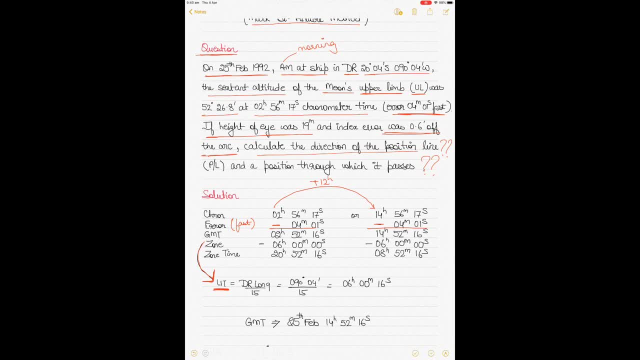 to a range of longitude. if your ship is within that range, that is the time it should be keeping. all the ships have the same time and and it helps to do business in world and to do business with the ports as well. all right, so anyhow, you can calculate longitude in time, or LIT, by dividing. 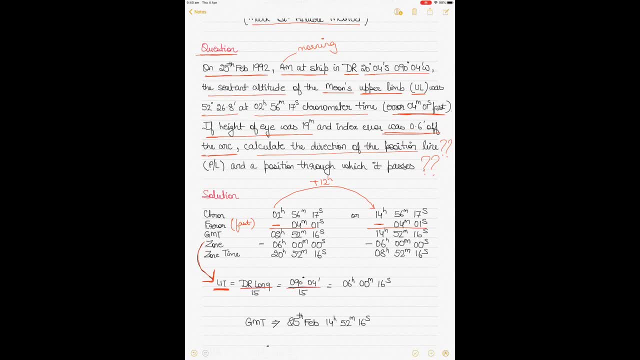 the longitude by 15. in this case it's 90 degrees 4 minutes divided by 15, which gives you 06 00, 16 seconds. so 06 hours 00 minutes, 16 seconds. this is the LIT now. LIT is always written in hours. 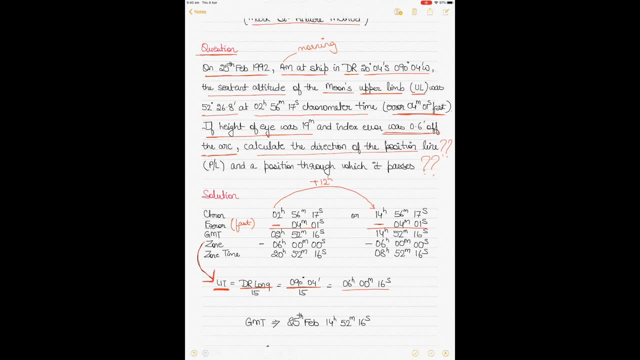 minutes and seconds and it can be not a round figure. but for zone it has to be a round figure, it has to be a whole number. so since the LIT is closer to 6, we will make the zone 6, and that's why you have the zone 6 here and you see a negative sign. the negative sign is because you 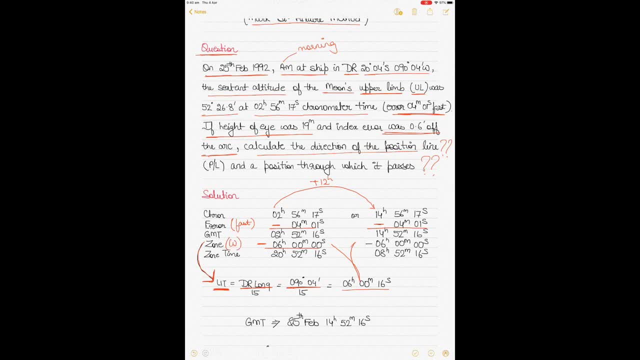 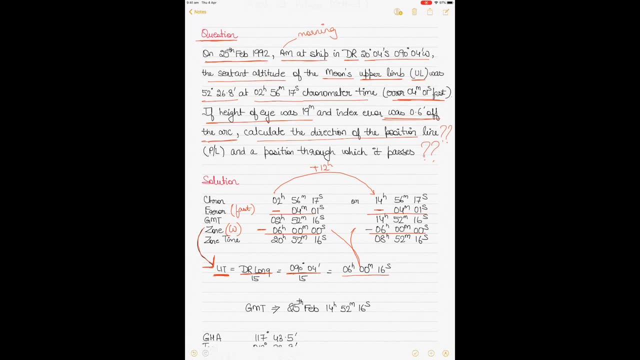 are in west longitude. whenever you are in west longitude, you will subtract your zone from the GMT because GMT is ahead of you, all right. so imagine yourself being in America, which is in west longitude, and GMT is the time at UK. the time at UK will always be ahead of you, all right they? 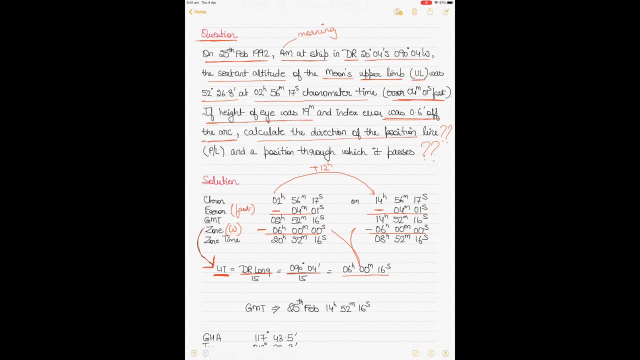 are, and so so. so similarly, if you are in east longitude- say, for example, you're in Australia or you're in India or you're in any of the Asian or Middle East subcontinent- then of course you are ahead of GMT because the time at UK is behind you. all right. so whenever it's west longitude, just subtract the zone. 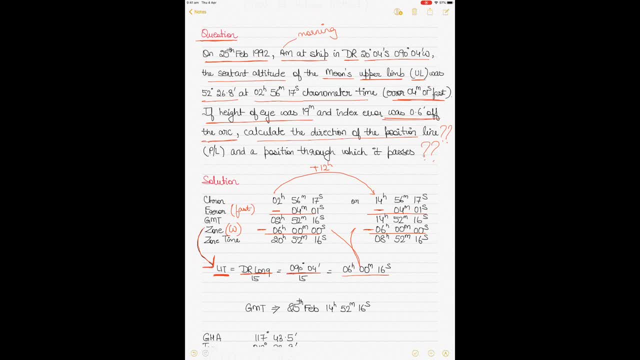 all right. so in case you are wondering in the first case, how did I subtract 6 hours from 2 hours? well, just add 24 to this and make it a bigger number and then subtract it all right, and then you get your zone time. your zone time is the time kept on your ship. 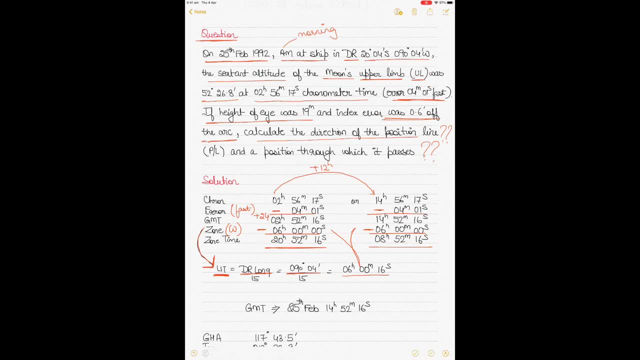 also, you get your zone time, which is the time kept on your ship, and then you get your zone time, which is also sometimes called ship's mean time or SMT. in the next case also just subtract 6 hours. so in one case you get 20 hours, 52 minutes 16 seconds, and in the other case you get 8 hours. 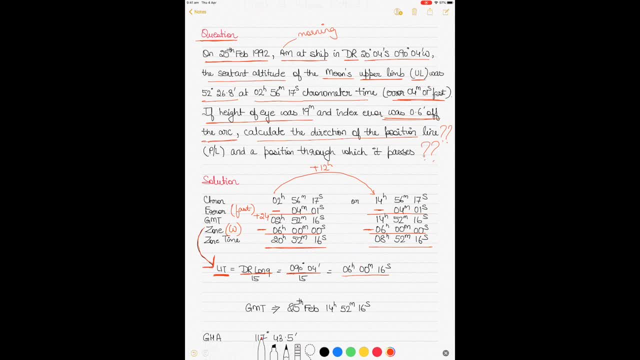 52 minutes 16 seconds of zone time. all right, so how do I know which is the correct zone time and resulting GMT? well, the hint in the question is that it's morning on my ship and it's 25th of February morning on my ship. out of the two zone times, I see only one time which says it's morning. 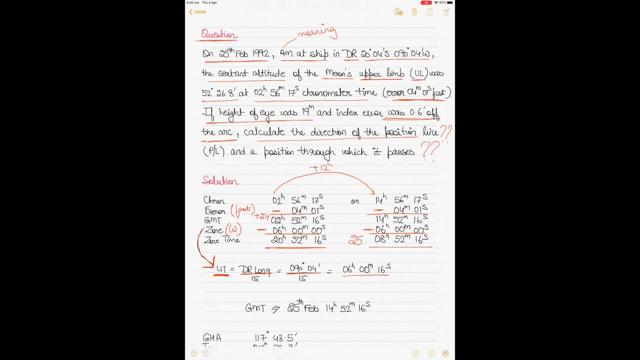 on my ship, which is the second case. so I will write it down and then I will write it down and then I will write 25th here and I know this is my case. I'll cancel out the first case. I don't need this one now. I have to figure out if the date of the GMT is also same after subtracting six. 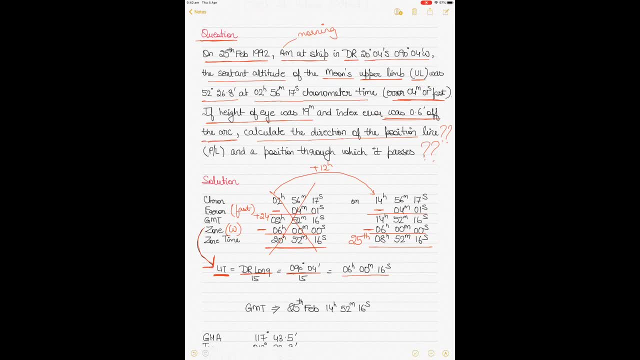 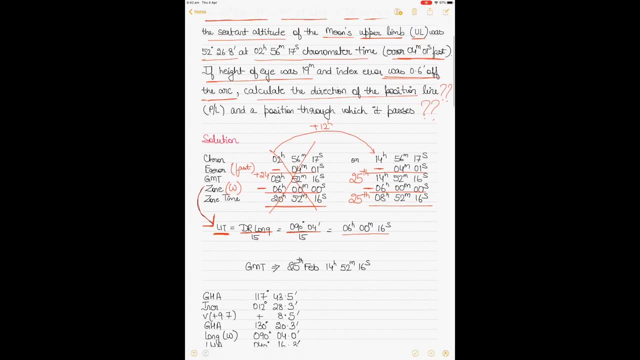 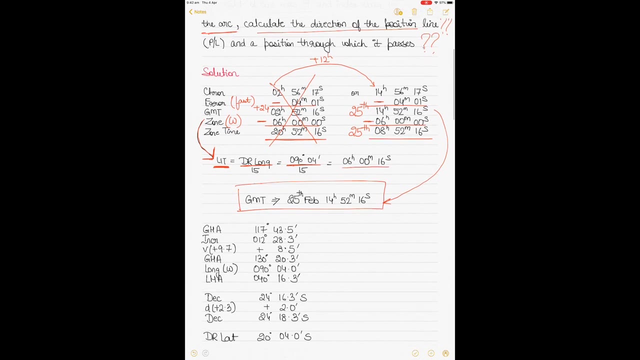 hours. well, yes, common sense says it, say it is. so the date at the GMT is still 25th, although they are about six hours ahead of the time on my ship. all right, that is why your correct GMT time is 25th of February. 14 hours, 52 minutes and 16 seconds. make sure you work with the. 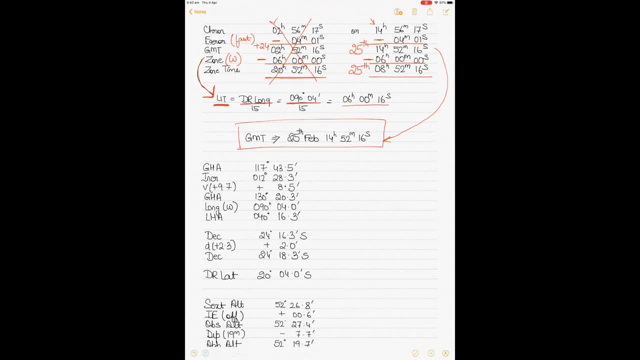 correct GMT time and not the zone time, because you have to use the GMT time to go into your nautical almanac and get the values from there. all right, so we'll go into the 1992 nautical almanac very soon and I will find out the GHA for 1400 hours, first, for 25th of February, then 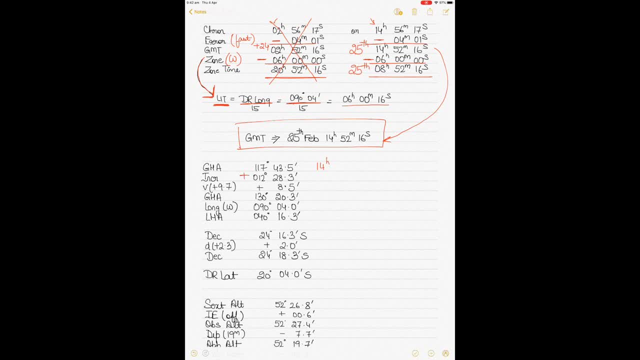 I will go into the increments pages. increments are always added. increment will be found for 52 minutes and 16 seconds. then I will find the V value, also from the nautical almanac, and then go into the increments page and find the V correction. all right, so I will go, not go too. 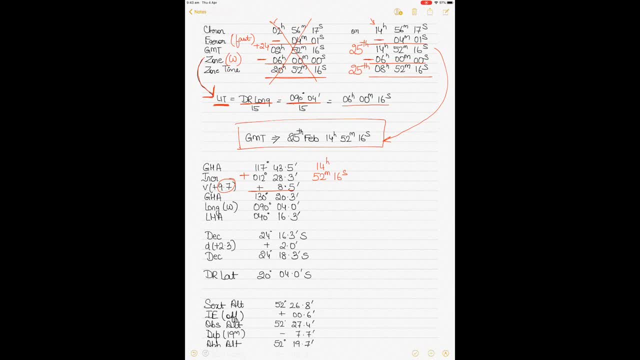 deep into it, otherwise you guys will get confused. so let's go into the increment, or rather go into the nautical almanac for 1992, and find out a few of these values, all right. at the same time I'll also show you where I can get my declination value from this value here and my D value as well. 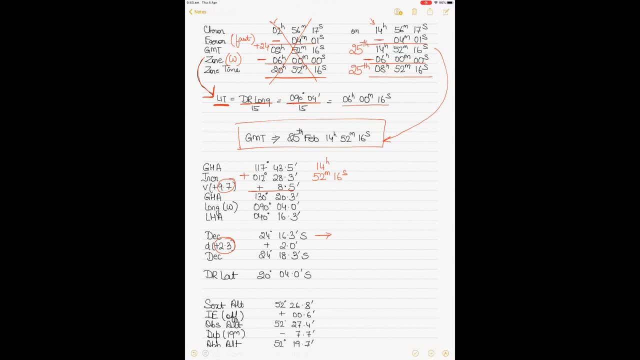 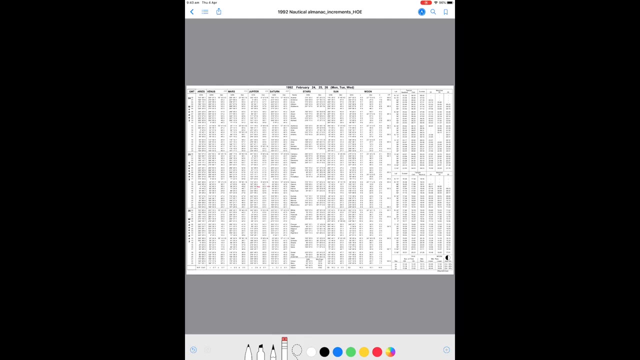 all right, so these are some of the values I can get from the same page. so, instead of going to and fro back and forth, that I go into one time and then show everything to you. all right, so let's go into nautical almanac. 25th February is the date, so I'm I've kept this page ready for you guys, so if I can show you here, 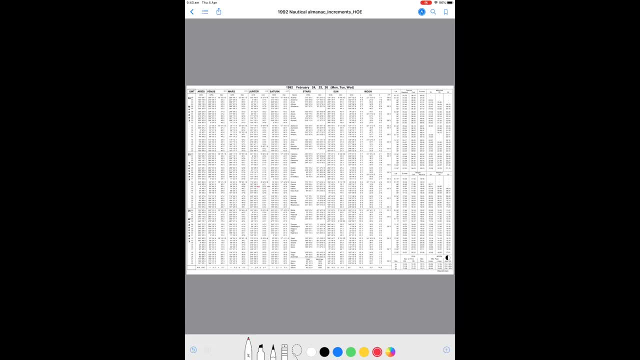 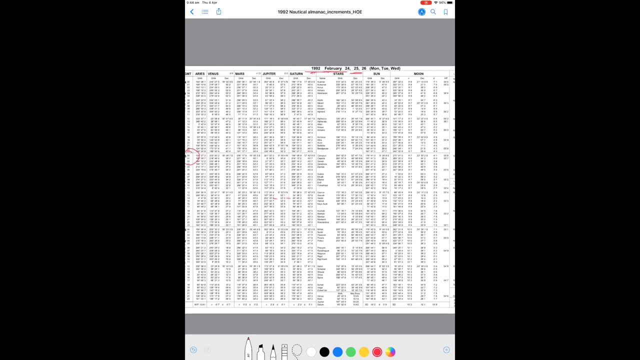 this is sorry. this is 25th of February. is here 1992, so this is 25th of February. I can zoom in a little bit so that I can show you both the. that's right if I zoom. okay, I think this is good enough for me. the time and the hour should be, and moon should be able to. 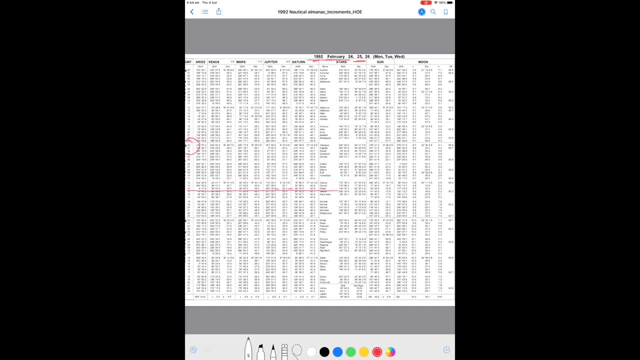 see. so 14 hours just go horizontal from here, so you can see you have to go further. this is Sun, right? so you can see. this is moon here on your extreme right hand side, all right, and if I erase this then I'll circle it again. so this is moon, this is moon, and then you can see the GHA values are given. 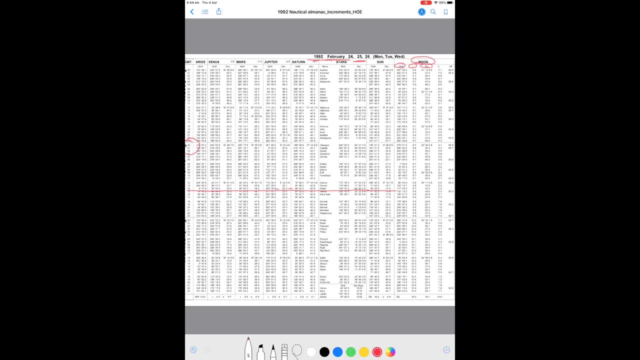 column. the V value is given under this column, the declination is under this column and the D values under this column. we'll also use the HP value, which is the horizontal parallax, but I'll come to that later on. all right, so for 14 hours, just find out what is. the GHA is, I think, 117, then this is the V value, this. 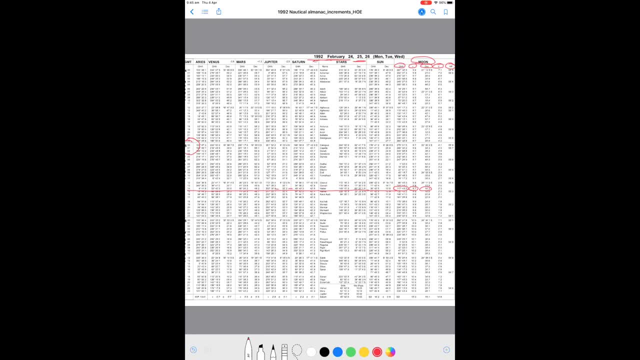 is the declination value: 24 degrees 16.3 South. and then this is the D value. and I'll come to the horizontal parallax of fifty five point four later on again, when I am resolving the sextant altitude. all right, so just note these values down. the reason I show you these values at one go. 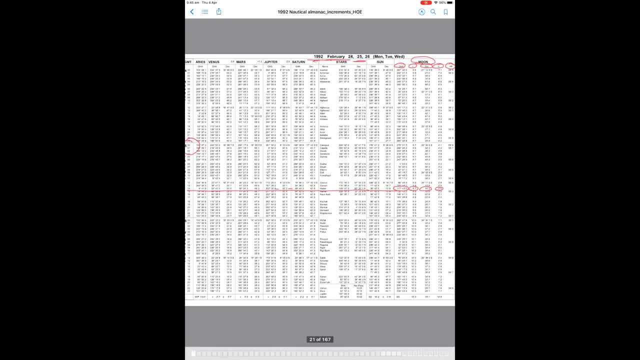 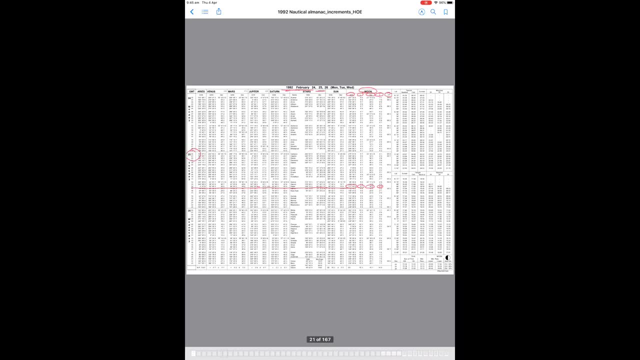 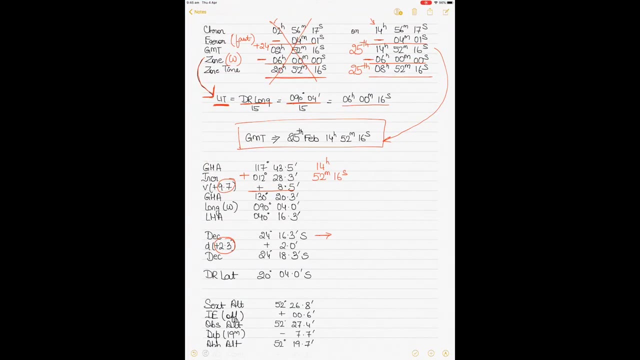 is because it's easier for you also, and easier for us so, not to go back and forth. I'll go into the increments page later on because I won't. you just make a note of these values and then I'll go back to the solution and show that these are the same values. I, everything all right. so 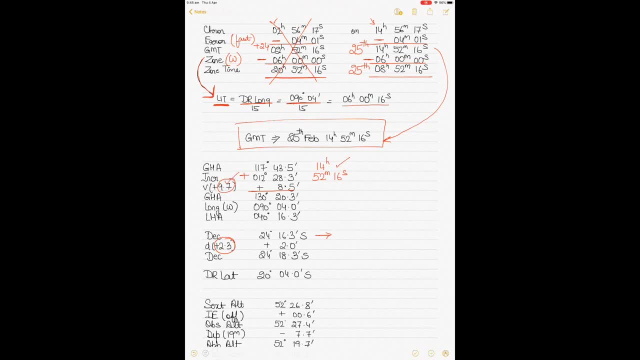 again. I have shown you the GHA value, I have shown you the V value, I have shown you the declination value and the D value. now I will show you where to get the V correction from and D correction from. all right, so the D correction is this value. here D correction is added. so if you note that the declination was, 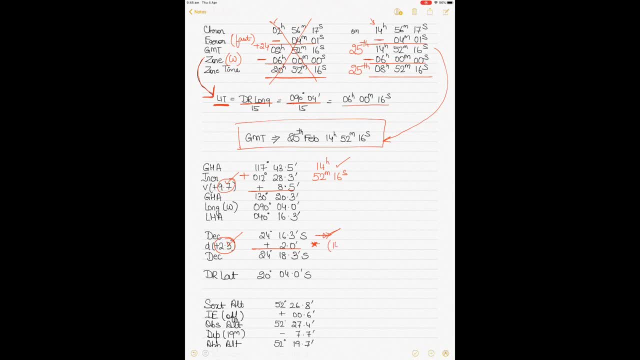 increasing, going from 14 hours to 15 hours. so from 14 hours to 15 hours declination was increasing. so you will add the D correction, all right, but the V correction is added based on the sign of the V value. so let's go back into the nautical almanac and go into the increments page for 52. 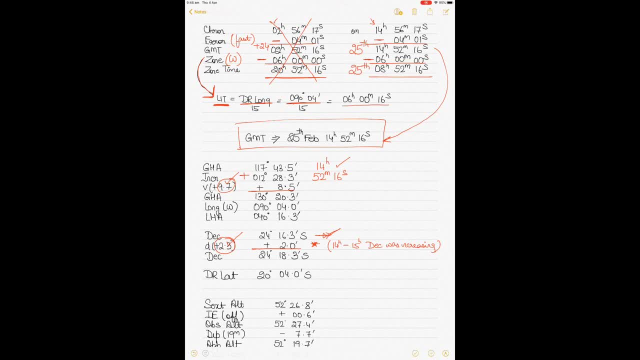 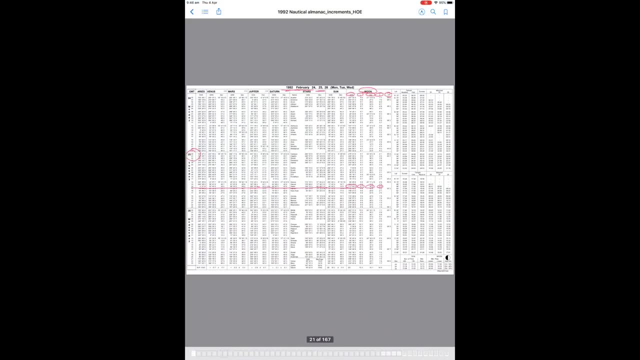 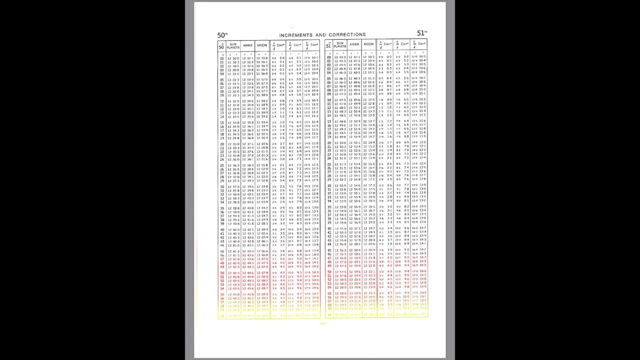 minutes and 16 seconds and for a V value of 9.7 and D value of 2.3, and then increment also, we'll find out all right. so 52 minutes and 16 seconds, all right, there you go. so I have page opened, but I'll erase some of this stuff for you. so you guys. 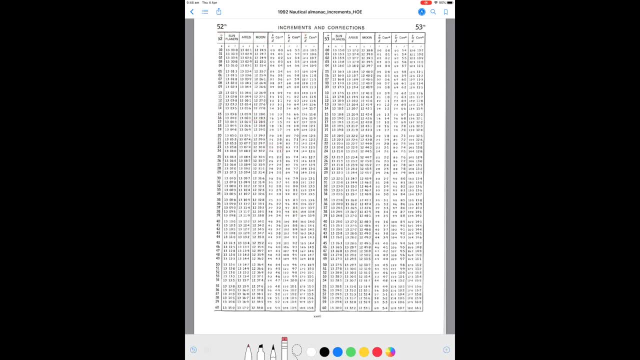 don't get confused. so 9.7 and 2.3 was here as well, so you can see the V and D values you get from these columns here. so for 2.3 of D correction, you get this correction of 2 and 9.7 of V value. 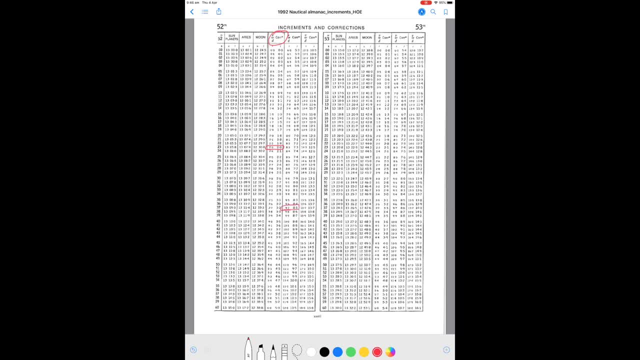 you get this V correction here: 8.5, right, and the increments is, of course, moon. is this column here? so for 52 minutes and 16 seconds is on the vertical column. 16 seconds is here. this is your increment: 12 degrees, 28.3 minutes, all right, so at 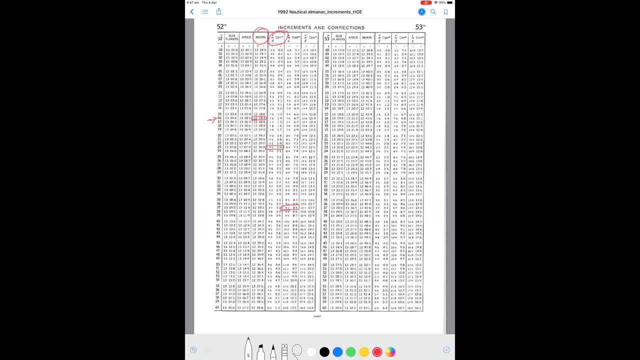 this point of time you can just pause this video and just have a look at this page and see where I got these values from. only when you're satisfied you can go back. but I'll keep going. otherwise the video becomes a bit long and I have been asked to keep the videos short, so I'll keep going, but you pause wherever. 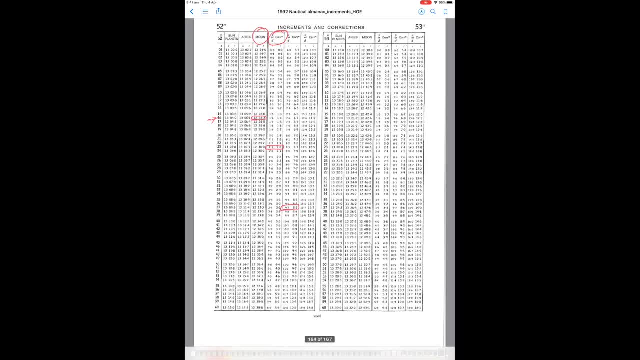 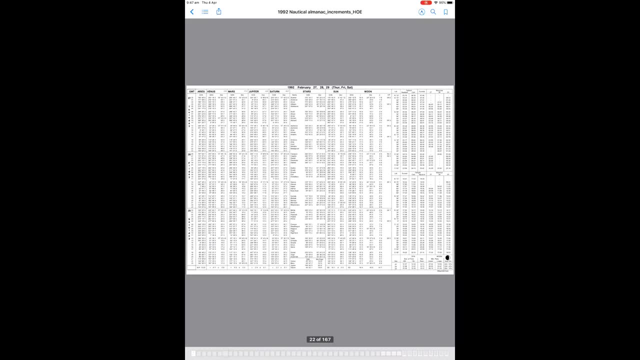 you think you know we are rushing through or you didn't get the idea. so I've kept this page for some time now, but I'll go back and into the 25th of February now, all right. so 25th of February is this page here, and if I 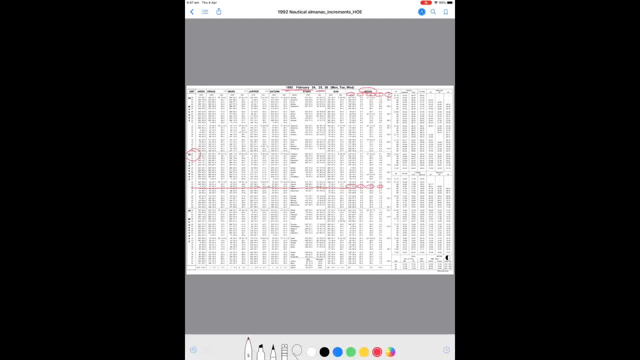 can show you about the declination. you can see the declination is increasing from 16.3 to 18.6, going into the next hour, right? that's why the D correction will be added. so I'll erase this and you can see, right. and also let me show you. 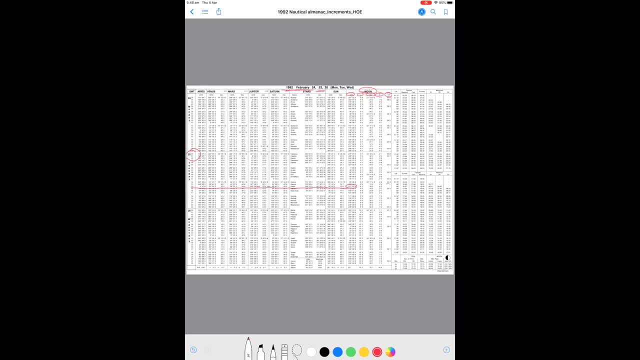 the horizontal parallax now, because otherwise we'll have to come back to this page. so the horizontal parallax is here: 55.4. so from 12 hours all the way to about 15 to 16 hours it will be 55.4. so remember this value of horizontal. 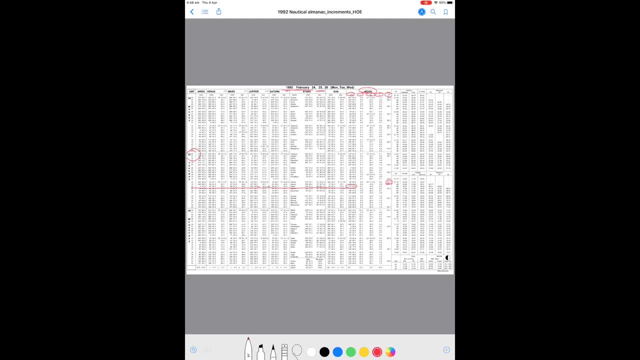 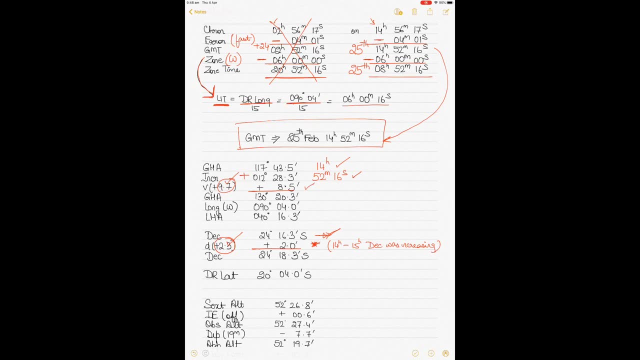 parallax when I use it later on. all right, so I don't have to come back to this nautical almanac anyhow. so I showed you where to get the increments from and the V correction and the D correction as well. right, so let's resolve the GHA. 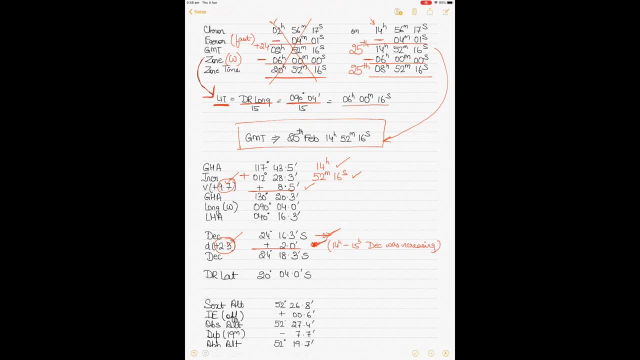 first. so I have resolved the GHA, I've added the corrections, I've got the GHA and then I've got my longitude of 0.9.5.. 0.04 minutes and longitude West. GHA is the best. that means GHA will be more. 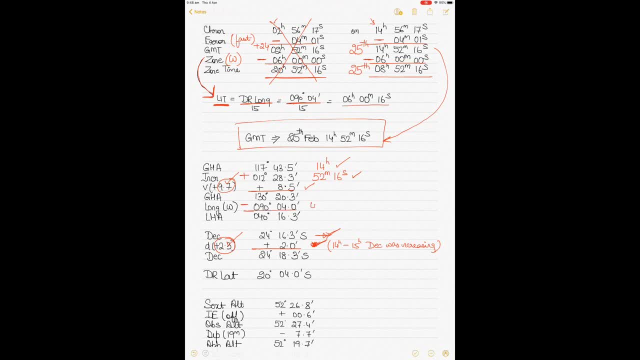 than LHA. so you will subtract the West longitude, so longitude West. this is a rule of thumb. longitude West, GHA, is the best, all right, compared to LHA. so GHA has to be more than LHA. so whenever you see this longitude, just subtract it from. 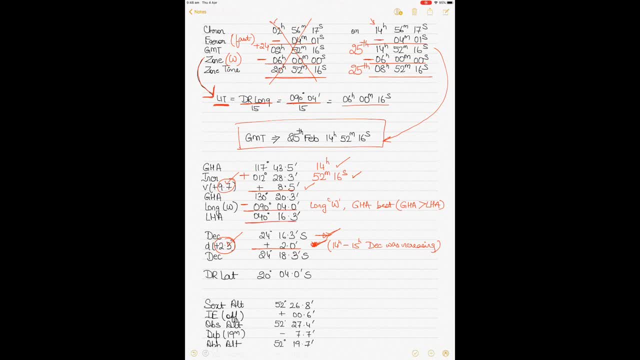 the GHA and that gives you the LHA. now you can name this LHA and you can name it West, because if LHA is between 0 to 180, it's West and if it is more than 180 to 360 degrees it is named East. 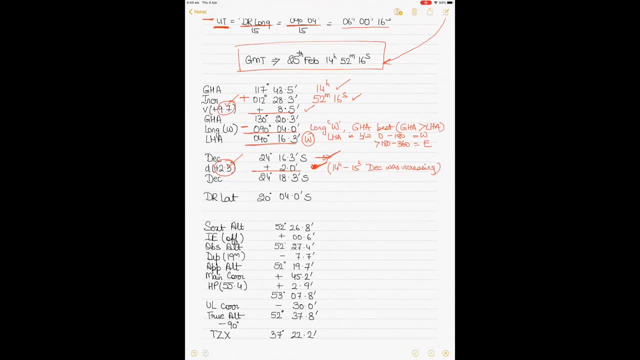 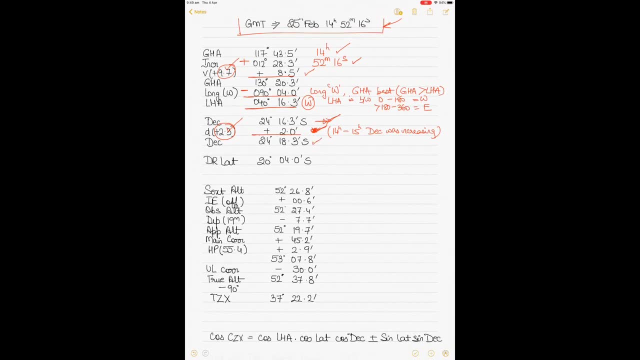 all right, so make a note of this rule of thumbs. it will help you understand how to name things when we go further into the question. all right, so I've got the declination as well. I have applied the correction and I have got the final declination as 24: 18.3 South. I have written down the DR lat as well, because 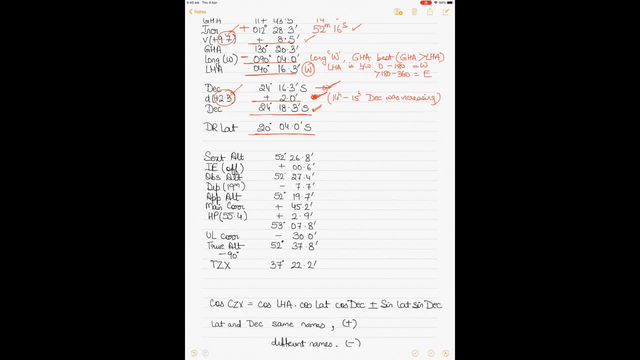 I'll be using this for reference later on in the question. let's resolve this sextant altitude. now the sextant altitude is given to us in the question. the index error is of the arc. whenever it's of the arc, you will add it. we add it into the minutes. we get the observed altitude, then we have to find the dip. 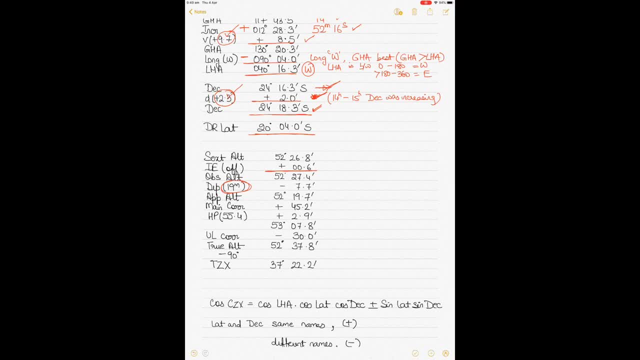 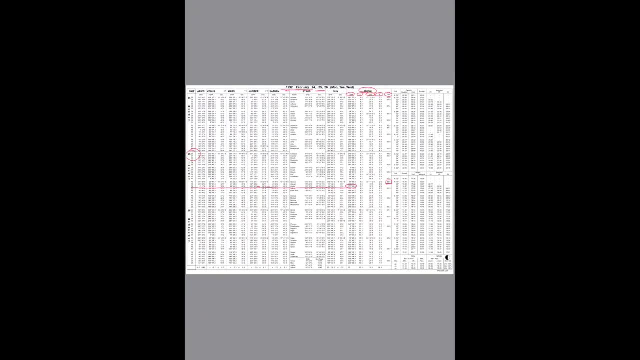 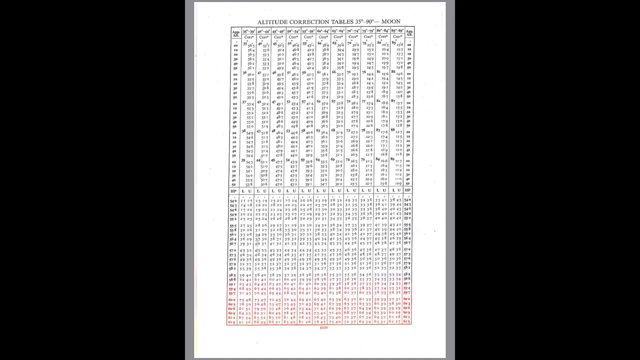 correction for a height of high of 19 meters. let's go back into the almanac and for what I will do is I basically use. I basically use these pages here at the end of the narticle almanac which are called altitude correction tables. 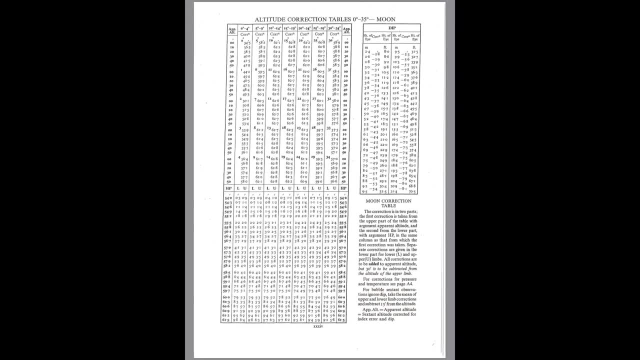 all right, these are called. these are called altitude correction tables and these are normally towards the end of the nautical almanac. all right, so you can see, for a height of i is here. this is dip. dip correction is also height of i. so height of i in meters, 19 meters is will. 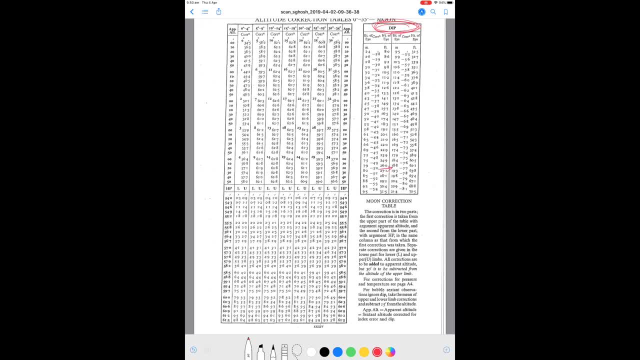 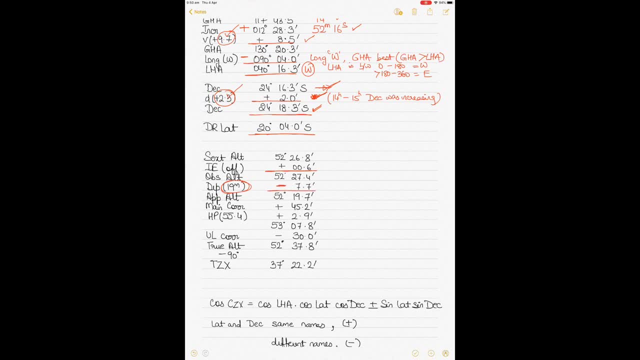 be lying somewhere between here. 18.8 and 19.3 should be minus 7.7. all right, so i'll go back and, as you can see, that's the correction of height of i minus 7.7. height of i correction is always negative. all right, once you subtract it, you get an apparent altitude. all right, so 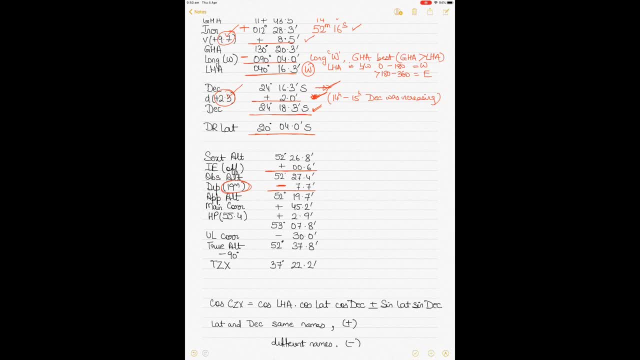 this app, altitude stands for apparent altitude. so you take this value of 52 degrees 19.7 and you go back into the tables from where i got my height of i from and you can find out the main correction and the horizontal parallax correction. so remember the horizontal parallax value i showed. 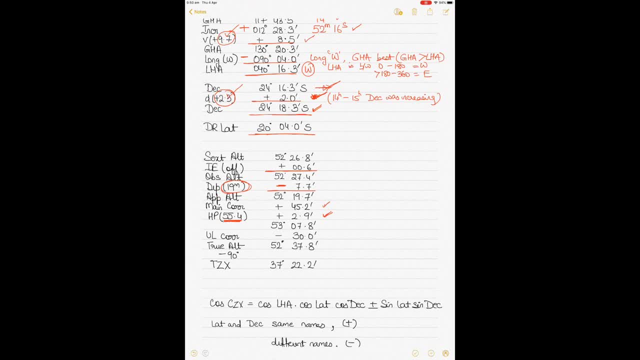 you before the horizontal parallax was 55.4. well, you use this value to find a correction, all right, and then you will add these corrections. so let me show you where to get this correction. so let me show you where to get this correction. so let me show you where to get this. 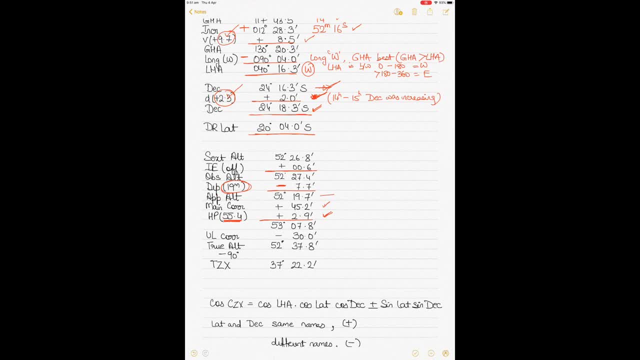 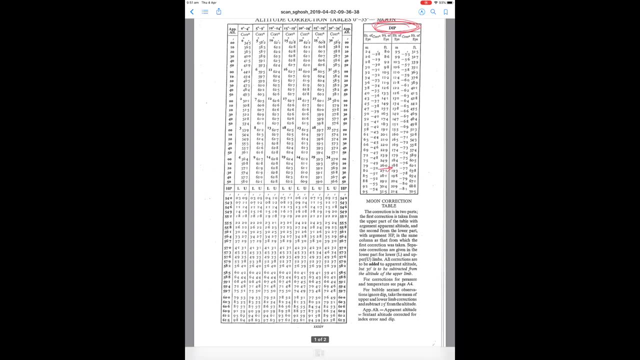 clingy particulared values from, so all you could do is remember the apparent altitude value of 52 degrees, 19.7 minutes. all right, so i'll go back into the same page. so you can see i have come back in the same page here, so the i'll go to the next page here. 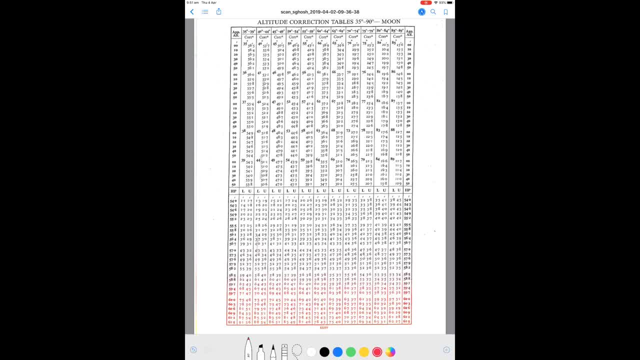 so for 52 degrees in 19.7. you can see the apparent or. these values of degrees are in the horizontal column here. this is the degrees one and this vertical column is minutes. so for 52 degrees 19.7, this is 52 degrees 19.7. 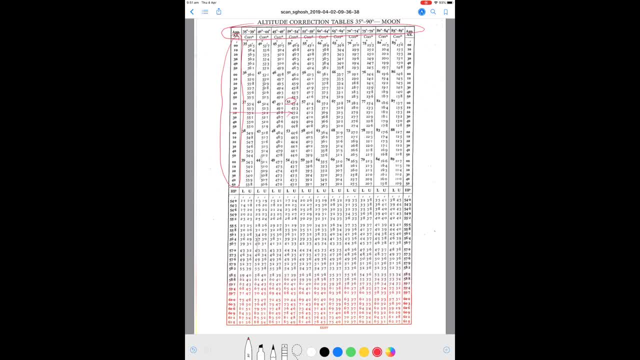 will be somewhere very close to 20, so your main correction will be 45.2 also. also, your horizontal parallax value is here for 55.4, which is very close to 55.5, and your moon's? it was moon's upper limb, remember. in the question it says it's upper limb. you go into the column here because this is. 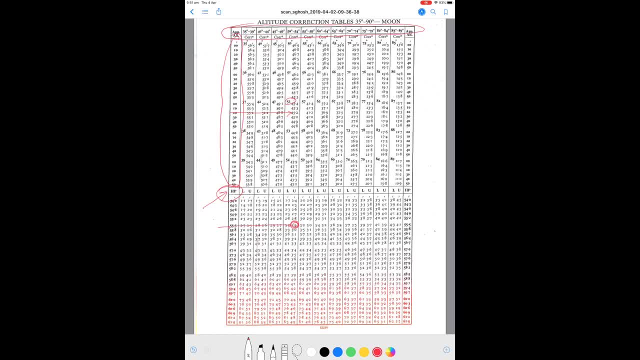 where your apparent altitude column is for upper limb. so l stands for lower limb. u stands for upper limb here, so you see the u one. because it's upper limb, you get a correction of 2.9. i take this correction, go back and that is what i have applied: 45.2 and 2.9. add the values you will get. 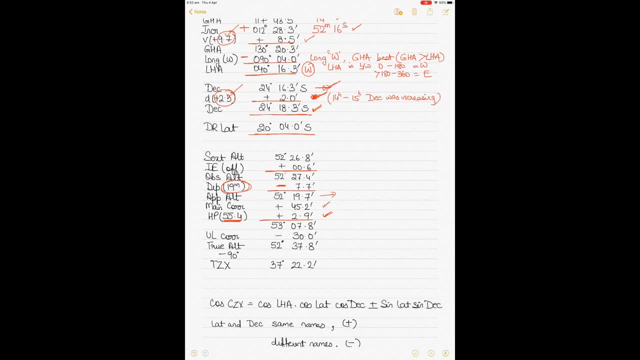 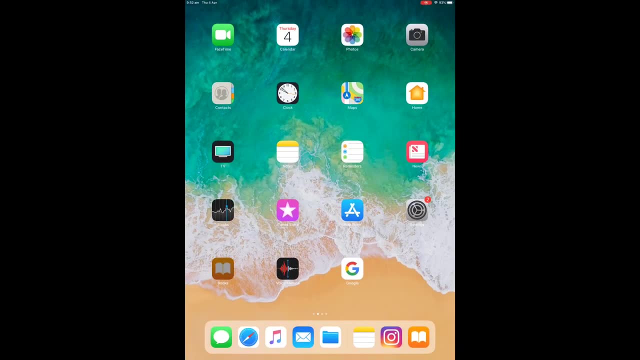 the apparent altitude corrected and then, whenever it is upper limb, you apply a correction of minus 30 minutes. all right now. this is also mentioned in the table. yes, if you go back into the tables you will see on the first page. sorry, on the first page you. 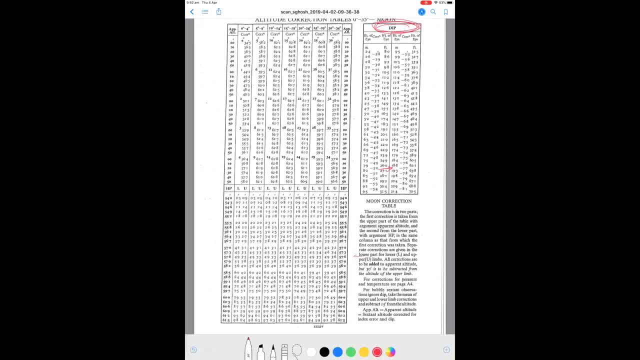 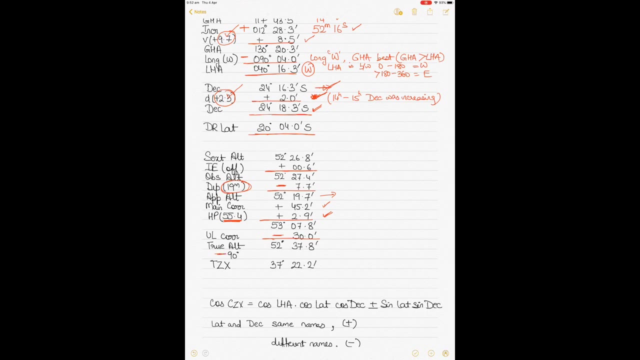 it says over here. all right, it says over here that if all corrections are to be had, the 30 minutes is to be subtracted from the altitude of the upper limb. all right, so just subtract 30 minutes and then you get your true altitude. then subtract the true altitude from 90 degrees and you get your true zenith distance. 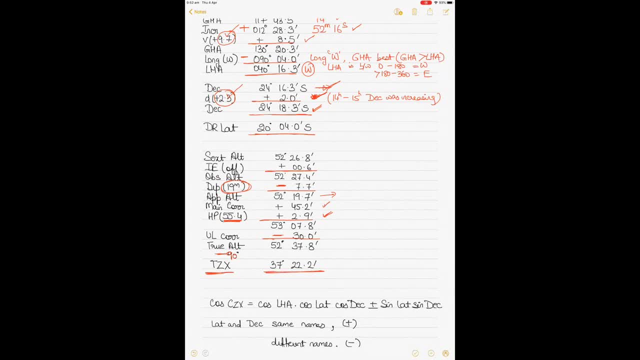 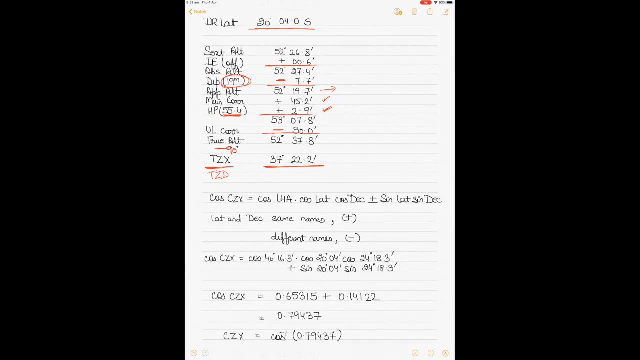 tzx. tzx stands for true zenith distance. in some books they also write it as tzd tzx. it is a same thing: true zenith distance. once you get your true zenith distance, you have to calculate something called the calculated zenith distance, or czx. czx stands for calculated. 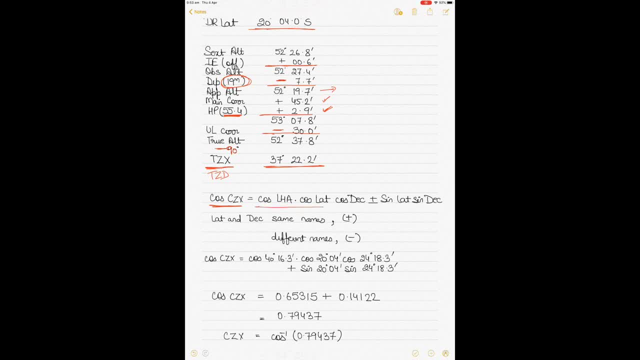 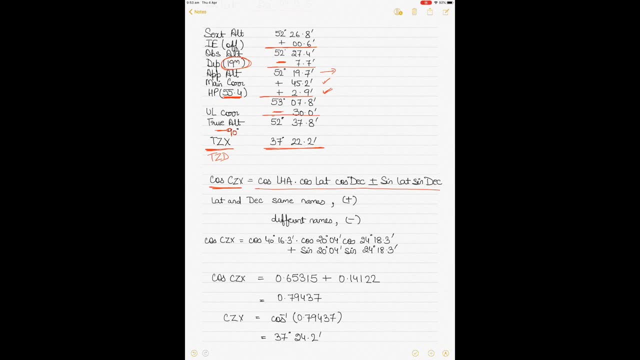 zenith distance, and you can calculate it by using the formula here on the scientific calculator. there are also other ways to do it, but we use a scientific calculator because these days everyone has a scientific calculator, right. and then you see over here, it says plus and minus, both. well, this depends on how many times you have to do the calculation in your 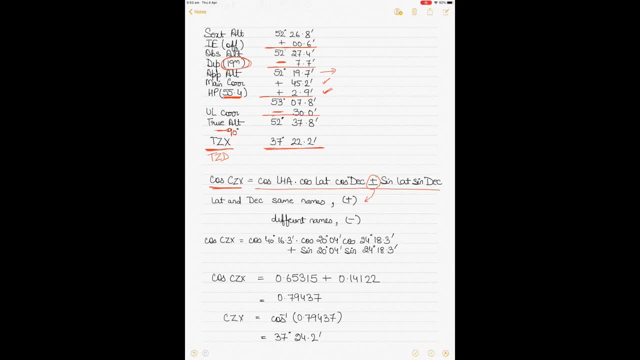 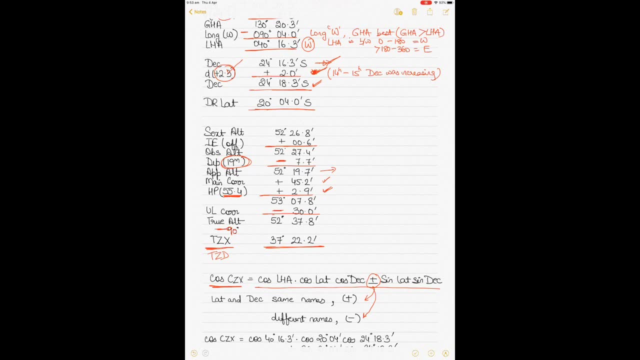 language, because obviously you have to do the calculation in other languages. so basically, whether your lat and dec are same names, then you will add it. if they are different names, you will subtract it. so in this case your latitude and declination are both south right, so you will add. 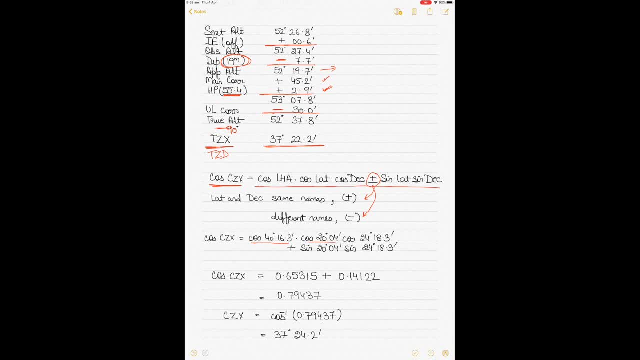 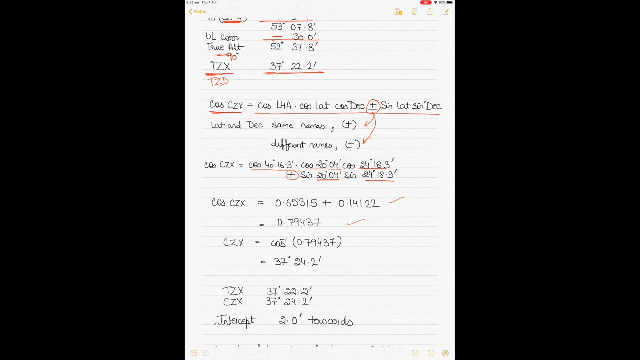 it simply put in the values of the LHA, the latitude and the declination, again the latitude and declination, and you will add it because the latitude and declination are same names, they are both in the both south. then you solve the equation. you can compare the values with the one that I 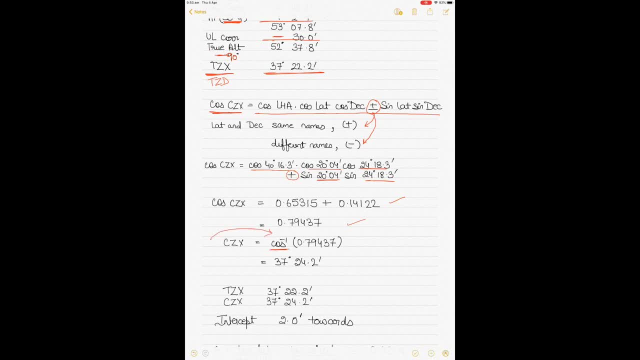 have written here and then take cos onto the other side becomes cos inverse. to get the Czx, I stick to five decimal places because it gives me reasonable accuracy. you can go more if you want. don't go less, because the more you go the better is the accuracy. and then you calculate this calculated. 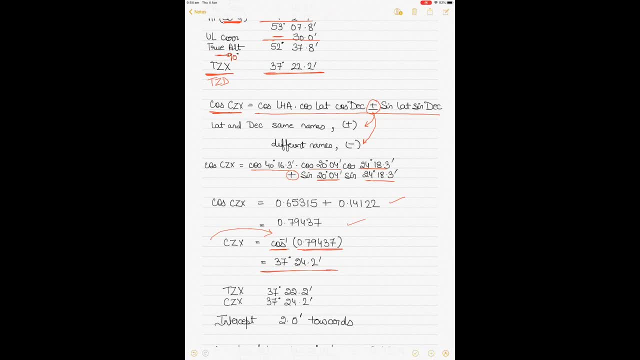 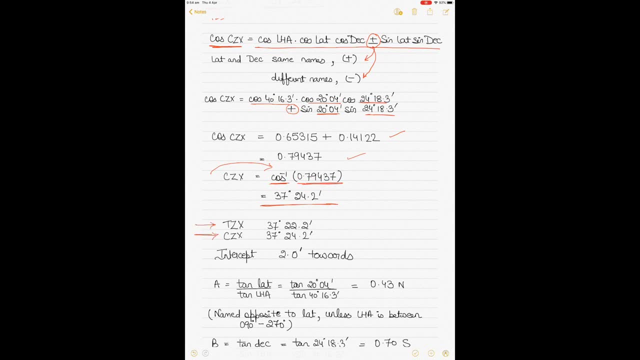 zenith distance, all right, which should be very close to the true zenith distance. then you can write down the true zenith distance here and the calculated zenith distance here. so the true zenith distance from above and the calculated zenith distance is what you have written here. so you have just calculated right. then subtract the bigger, subtract the smaller from the bigger. 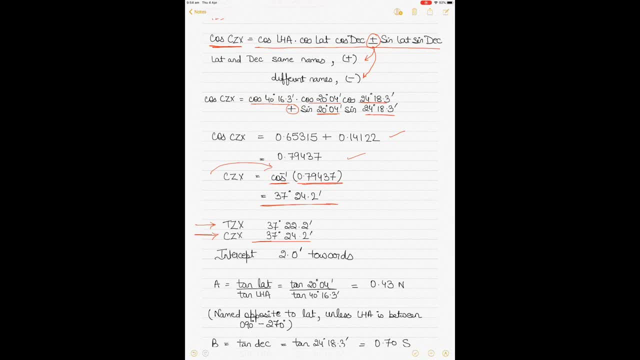 all right. so in this case Czx is bigger, so you subtract Tzx from Czx, you get intercept of two minutes. now this difference between Tzx and Czx is called intercept and that is two minutes. and then I have named it two words. that means it's two words. is celestial body. how I have I named 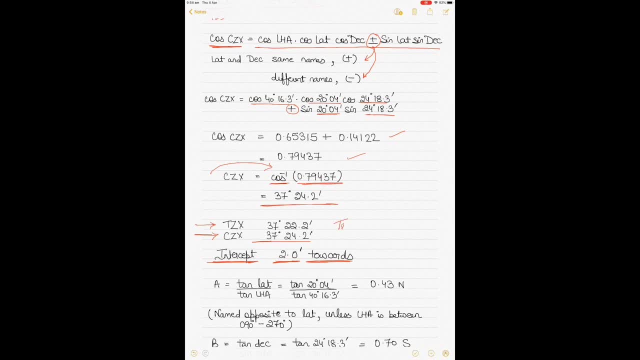 it words. well, there's a rule. if you can remember this rule, it says true, and if tiny, then it is two words. that means: if the true zenith distance is less than the calculated zenith distance, then it is two words, all right. if true zenith distance is more than calculated. 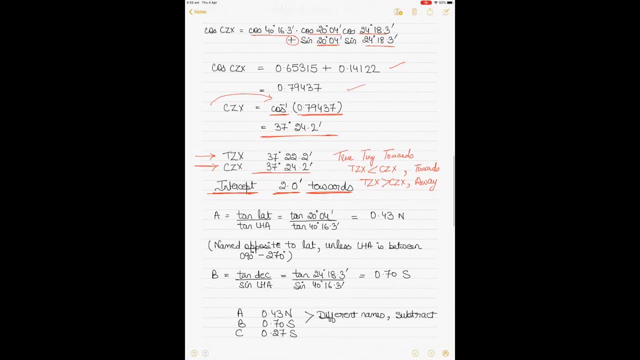 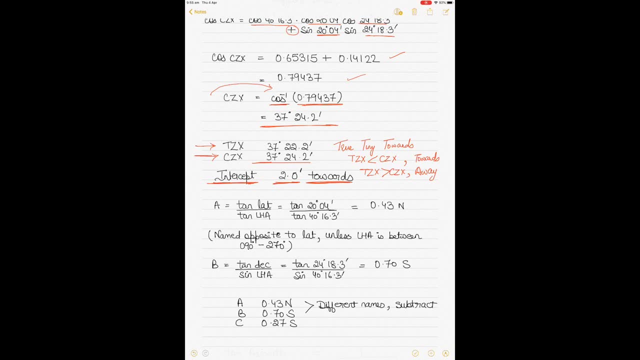 zenith distance. it is away all right now. in my staggered videos on staggered observations you can see how I have applied this rule of two words in a way. I will not go into all that in this video here, so if you don't know what two words and two words are, then you can see how I have applied this. 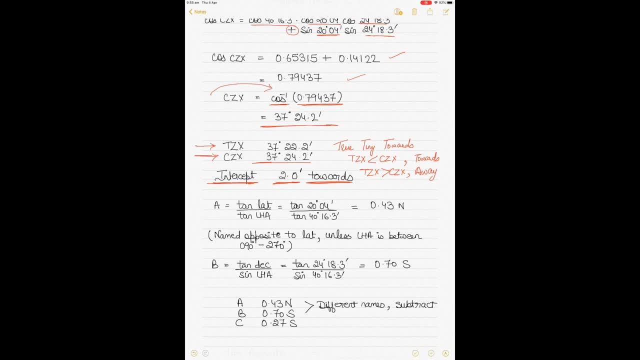 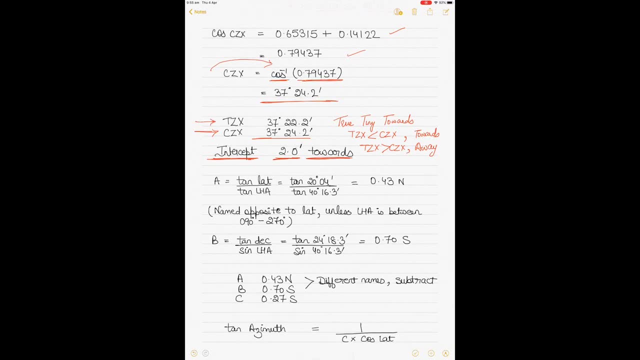 away means and how it all gets involved into actual plotting of the ship's position. please watch my video on staggered observations and you will see how it is all applied. all right, I'll continue. now that I've calculated the intercept, I need to calculate the position line, so to 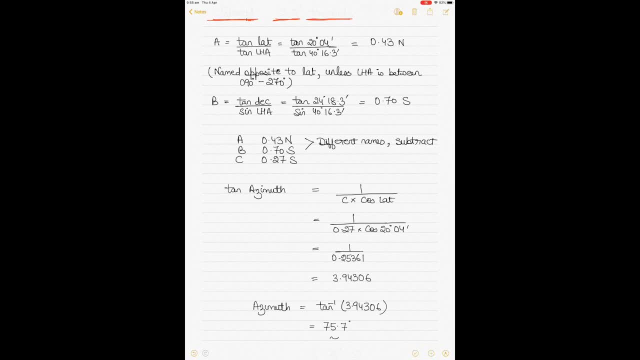 calculate the position line, I have to calculate the bearing. how do I calculate the bearing? well, I can create components of a by dividing tan led by tan, LHA, simply putting the values in the equation here and get write down the value, so the value you will be getting in the calculator. 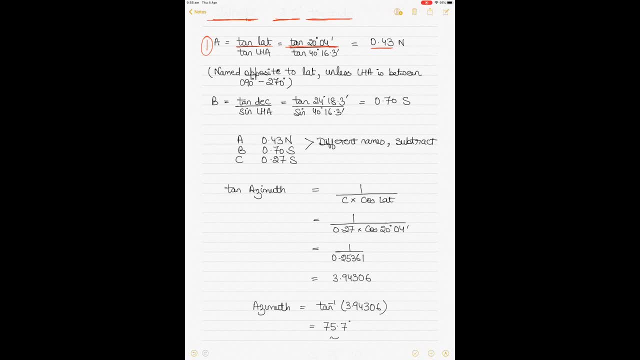 is 0.43. in case you get a negative sign, please ignore the negative sign. all right, ignore the negative sign, simply writing the value here, and then you have to name it. in this case, I have named it north. why? because it is named opposite to latitude, unless LHA is between 90 and 270, since 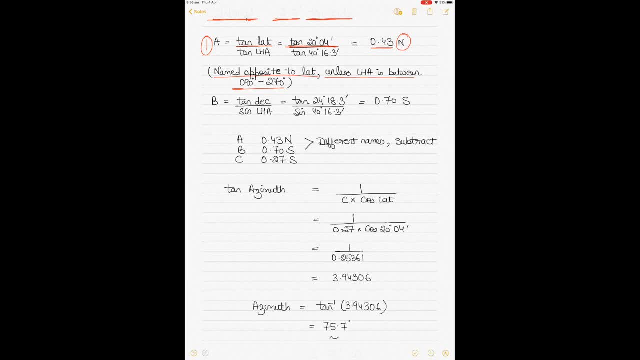 your LHA is not between 90 and 270, you will name it opposite to latitude. low latitude is south, so you name it north. then you calculate component of B by dividing tan of declination by sine of LHA, simply putting the values again. again, if you are getting a negative sign in the 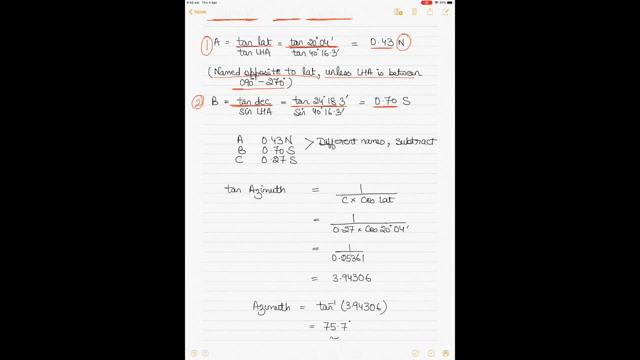 calculator. ignore the negative sign. just put in the value. you might get 0.699 something. just make it 0.70. I stick to two decimal places here. you can go more if you want to, all right, but remember to ignore the negative sign. don't include the negative sign here. these values are always. 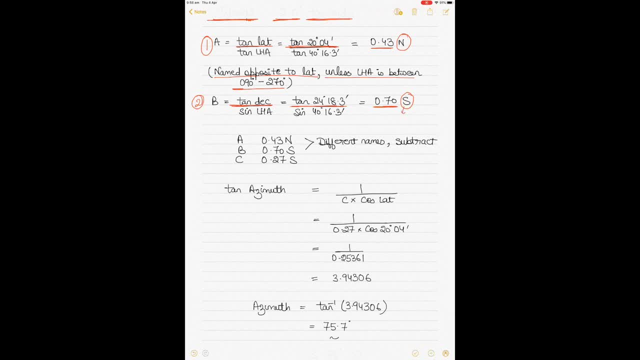 positive. and then you. I have named it south. why? because this is named same as declination. all right, so your declination is south, you will name it south. then write down the A and B values here. the rule is, if they are different names, you will subtract it. if they were same names, you would have added it. in this case they: 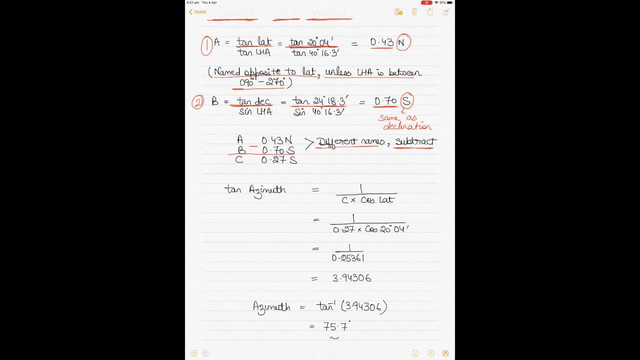 are different names. one is north, one is south. so you subtract it. just subtract the smaller number from the bigger number. don't worry what is written above. C values are always positive. they are negative, negative. all right, so you get 0.27 and then you get the name from the name of. 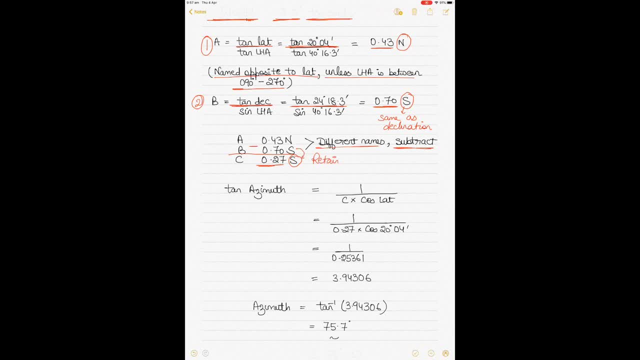 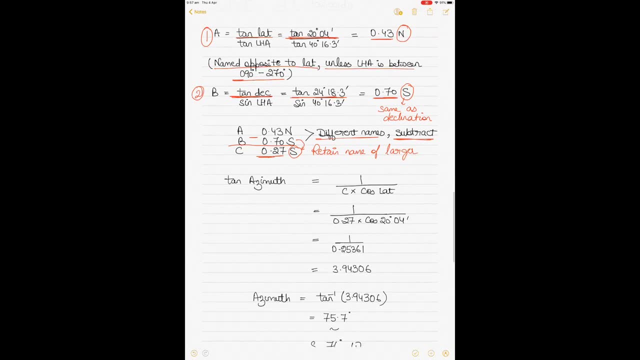 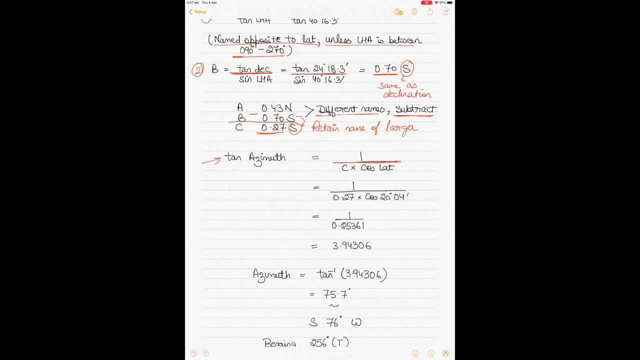 the larger. in this case south was larger, so you retain the name of larger, which in this case was B, which is south, so you will name C south. then you calculate the tan of azimuth using the formula 1 divided by C times cos of lat C, you have got from above as 0.27. 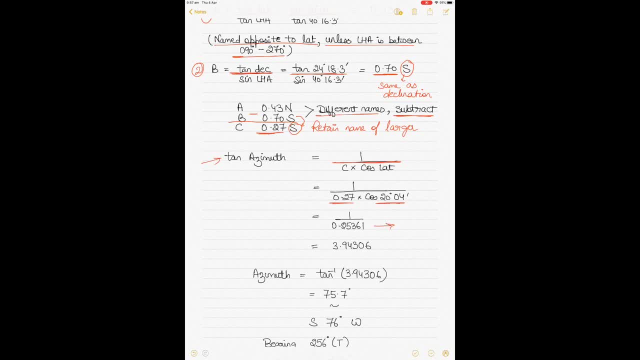 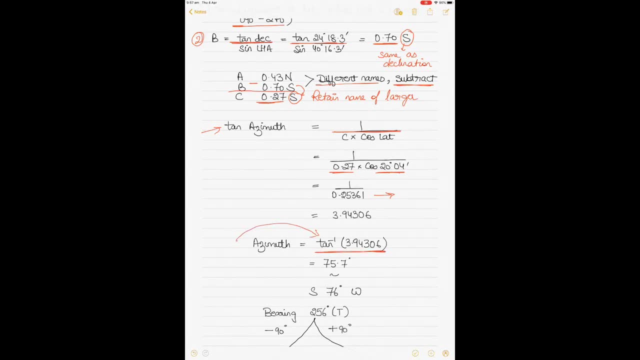 latitude. you know it's given in the question. solve the denominator first, then divide one by it, then take tan to the other side, becomes tan inverse. again, I have stuck to five decimal places. you can go more, don't go less, and you will get the azimuth of seventy five point seven degrees. 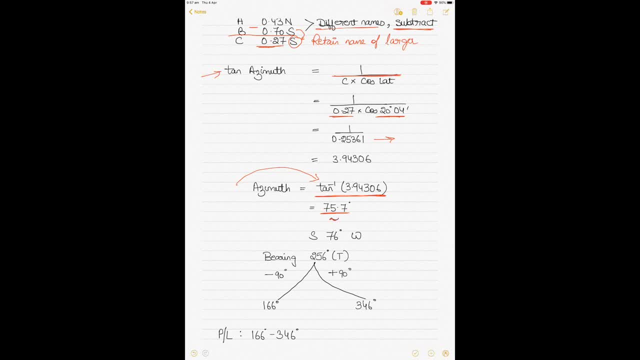 which, for practical purposes, I round it off to the nearest number, which is seventy six degrees. you can continue with seventy five point seven. it's still correct. some books continue with decimal, some books they round it off because sometimes bearings need to be plotted on the chart and you can't plot a bearing of seventy five point seven. all right in both the cases.